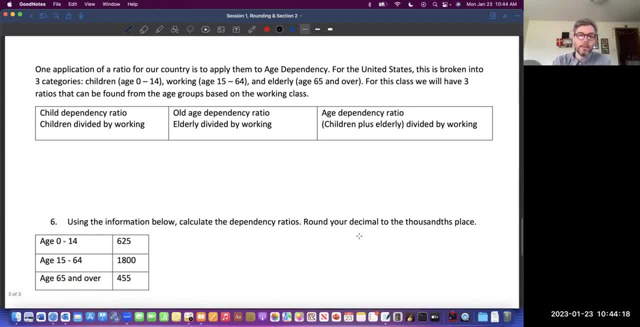 Now this is confusing. So child dependency ratio, old age dependency ratio and age dependency ratio is most likely going to be the most difficult thing to comprehend And of course it's coming at the end, but hopefully I can explain it clear enough. 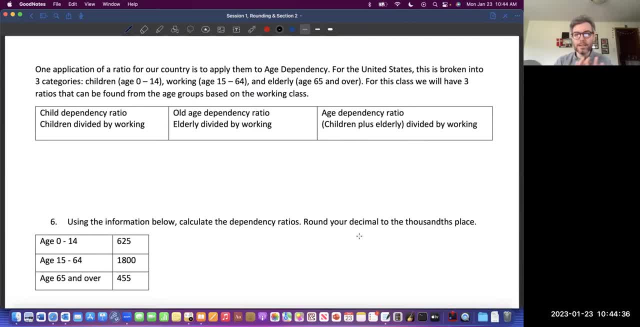 So child dependency ratio. this all has to do with- let me write this- this all has to do with working age. Okay, this all has to do with working age. So the idea is the denominator. what we're going to divide by is the group that is of working age. And this book will define it. working age is 15 to 64, though in reality that number, at least for this country, has kind of shifted. So people start working a little bit later, but then they finish- they don't quite retire- at 64.. 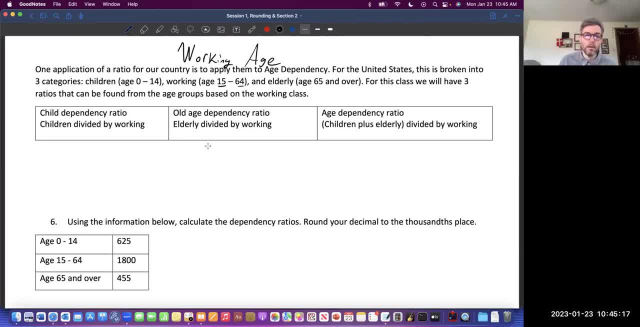 So it's kind of been shifted. That's what we notice more in reality. But in this class we consider 15 to 64 at the working age. Okay, 0 through 14 is considered childhood and 65 and older would be the elderly, the retired, that kind of thing. 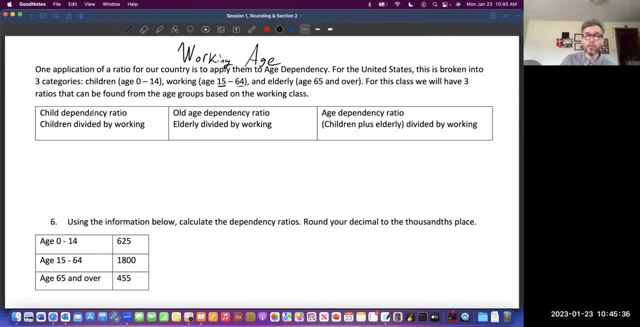 So child dependency ratio is the group, is this group of this ages and you're going to take children Divided by the working, The old age dependency, that ratio, this is going to be the elderly divided by the workers, And the age dependency ratio is the children plus the old age. 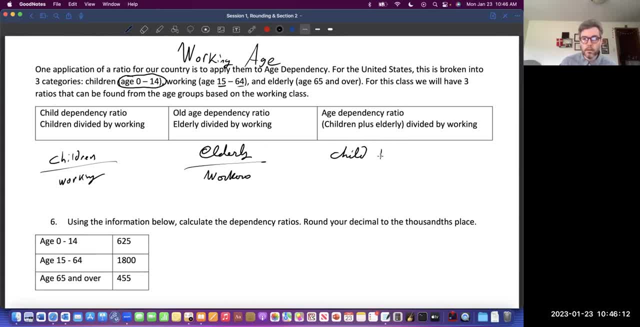 Okay, Child plus Elderly, divided by the workers. Okay, Please note, We do not divide by population. Okay, We're not dividing by the population, We divide by the workers. Okay, With this dependency ratio, we're dividing by the working age. 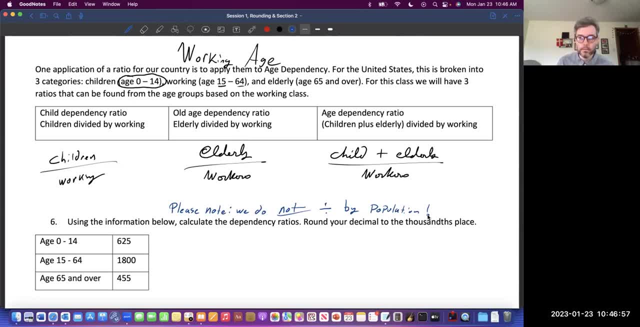 We are not dividing by the population. Okay, In other calculations in this class we will be dividing by the population Like per capita. We're going to go over per capita next time, But this time we are not dividing by population. 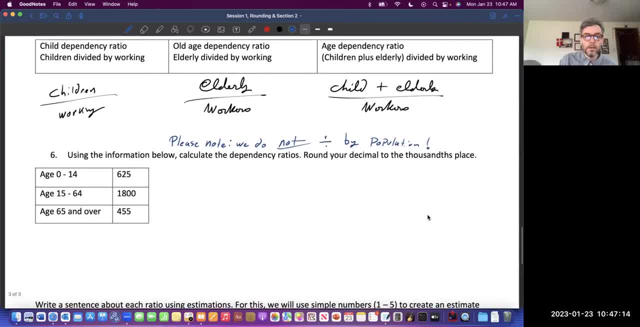 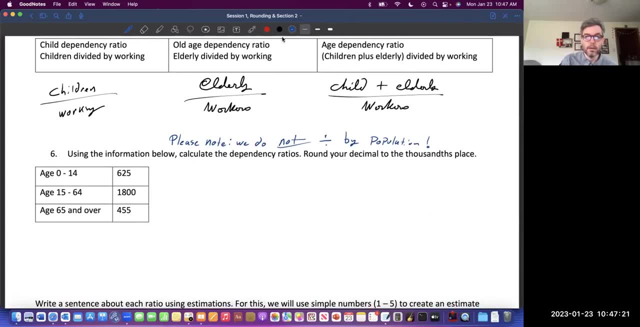 We're dividing by the working age. Okay, So let's do a problem Using the information below: calculate the dependency ratios and round your decimal to the thousandths place. Okay, Let's do that. So let's do the child dependency ratio first. 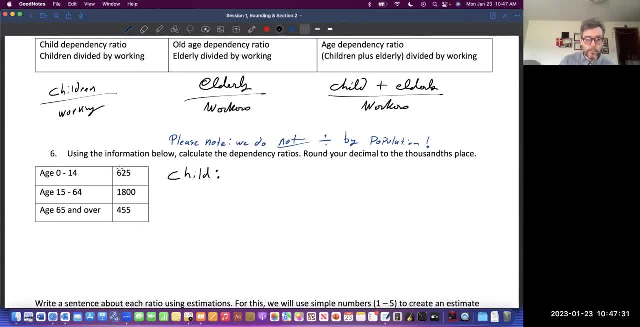 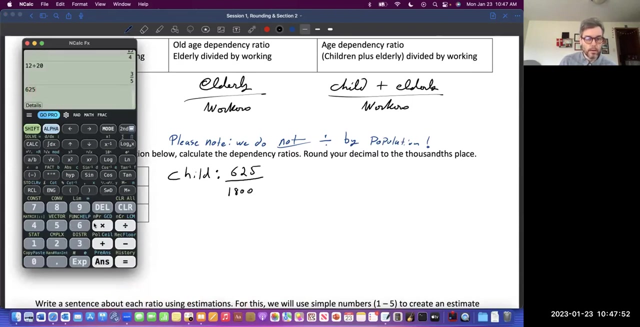 Okay, In this group of information there are 625 children And the working age is 18.. Okay, Now, as a decimal, round it to the thousandths. Hopefully you were able to see my calculator, But if you can't, the only thing I'm doing is dividing that. 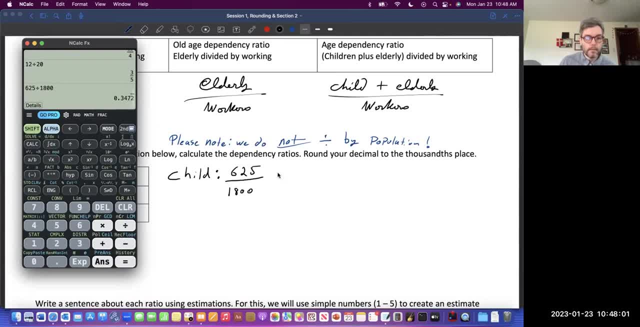 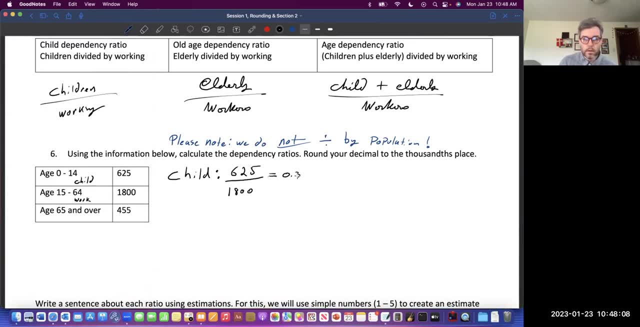 Okay, Convert So 3472.. 3472.. And we went around to the thousandths place That would be here. So that would be equal to 0.347.. Okay, There we go. Now let's do the old age dependency. 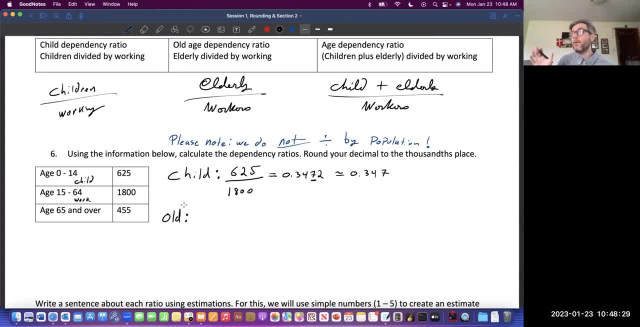 Let's see Now, if you're over 64 years old and you're listening to this, am I calling you old? No, I'm not calling you old, But that's what they determined it. Okay, The name. Let's see. 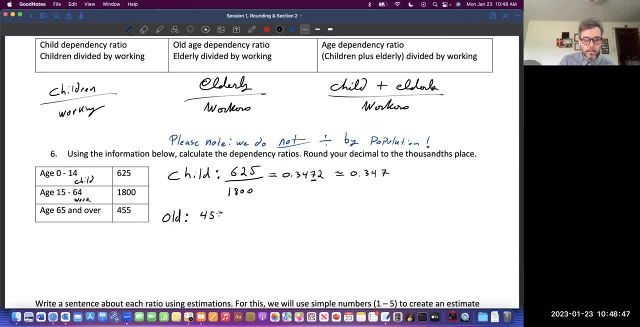 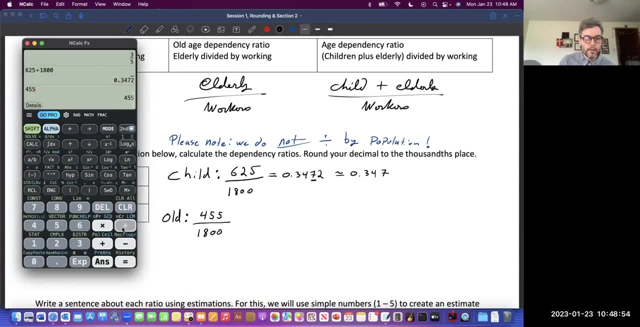 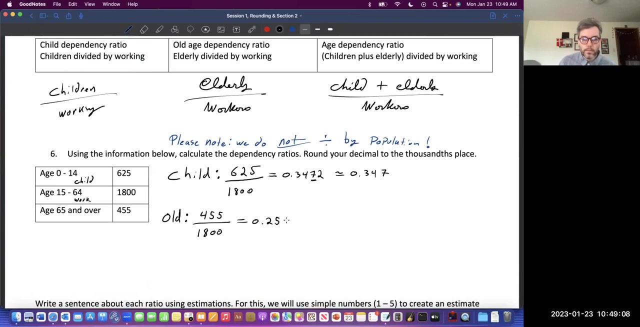 We have 455 of those people divided by 1,800.. Okay, So let's see what happens: 455 divided by 1,800.. And 91, 360, 25, 27.. Already forgot 25, 27.. 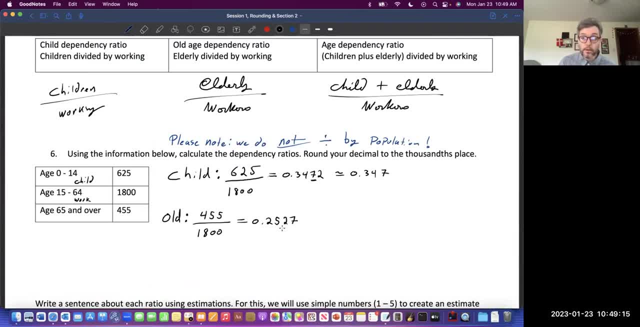 Yeah, All right, We went around to the The nearest thousandths, So that's that 2.. We look to the next digit, That's a 7. So that 2 is going up 0.253.. 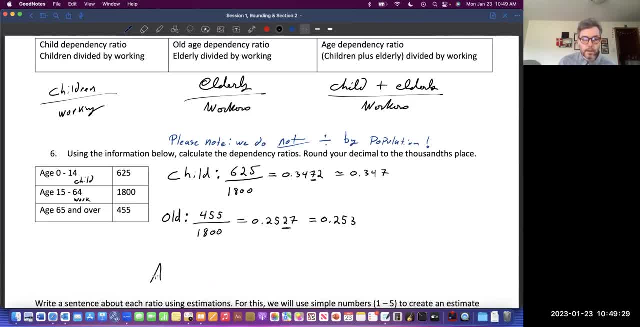 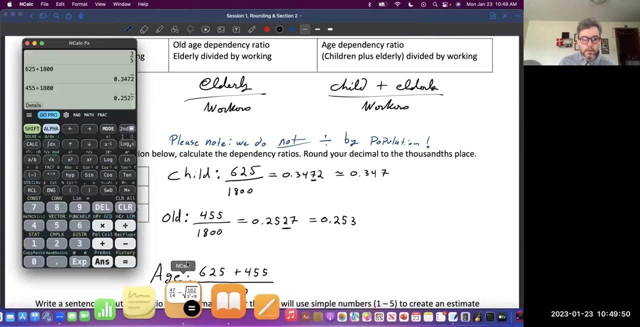 Okay, Now we're going to do age dependency ratio. This is where we add those two. We add the 625 and the 455.. Okay, Okay, the people dependent on the working age: 1,800.. Okay, let's do it 625 plus 455 and then divided. 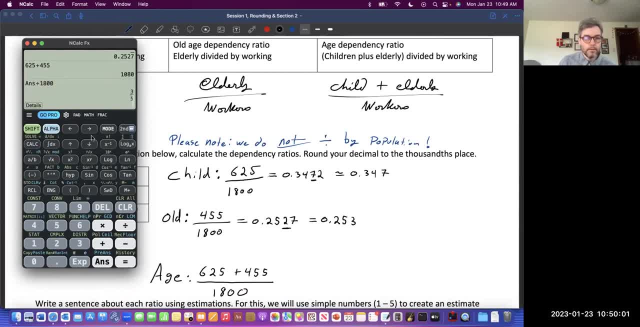 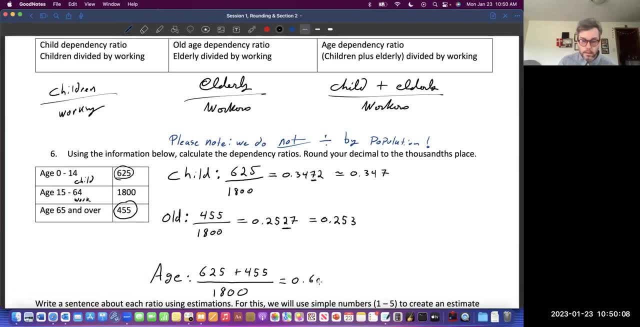 by 1,800.. Read this: 0.600.. Okay, All right, Age dependency ratios. Tricky, tricky, tricky. I mean they're easy. if you know what to do, There's just little steps. I mean, if you know what to do, it's not that bad. but it's all about knowing exactly what. 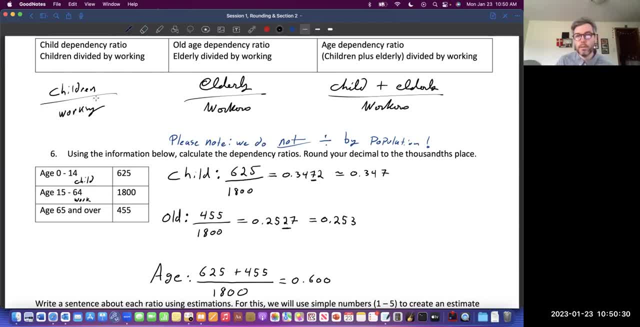 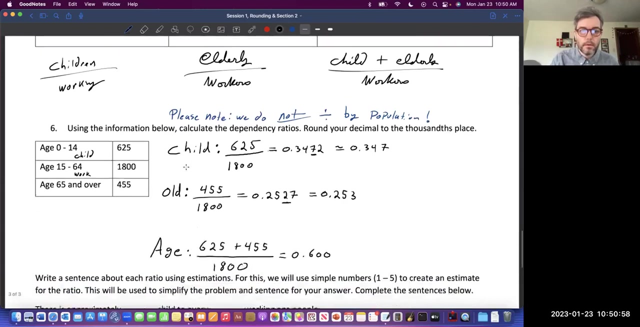 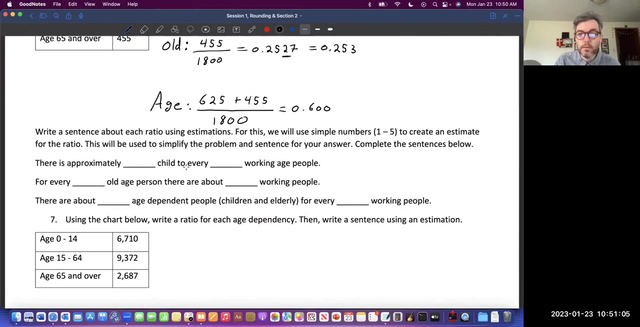 it's asking you to do. Are there any questions about these age dependency ratios? Any questions about that? I will post these notes later today in case they are helpful to you. Any questions about that? Okay, Write a sentence about each ratio using estimations. For this we will use the simple. 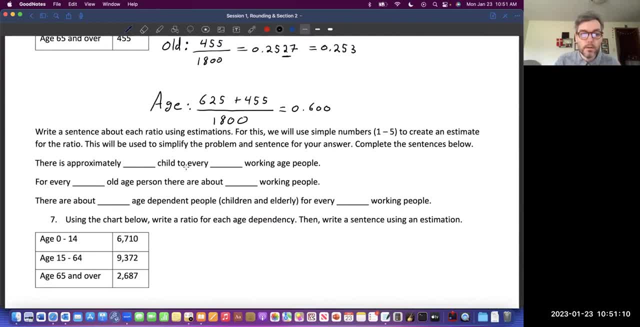 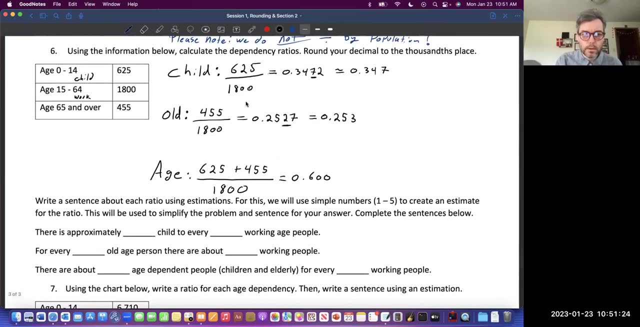 numbers 1 through 5 to create an estimate. This will be used to simplify the problem and sentence for your answer. Complete the sentences. Look, there are approximately blank children for every blank working age people. So, oh, there is a question. Are these in the textbook? Oh, so, are you asking. is this? 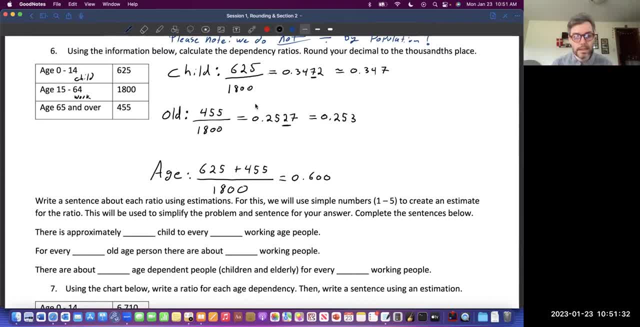 worksheet in the textbook, Caroline? Is that what you're asking? I think it is, So this is not in the textbook. So this is like what I'm working on right now. This is like a consolidation of section two. This is like a 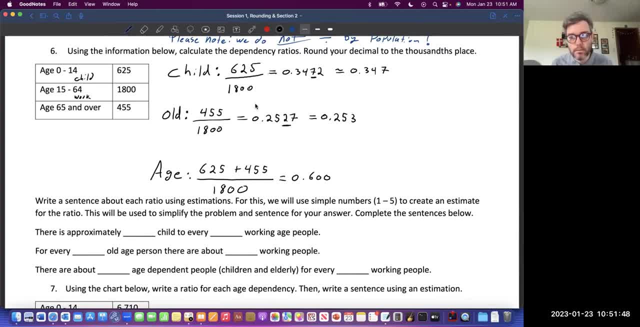 Boiled down. This is the minimum of what you would need to know. okay, Okay, Thank you. Yeah, Yeah, Great, But I will post this. I will post this after class, So you will have access to these notes after class. 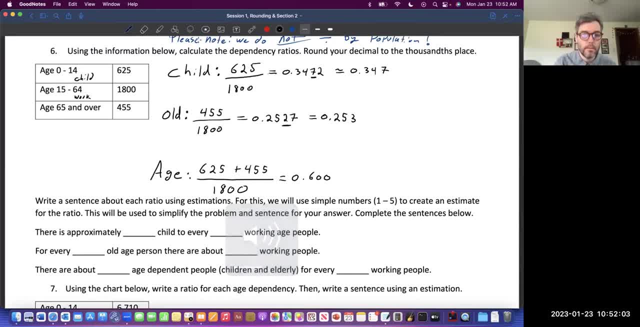 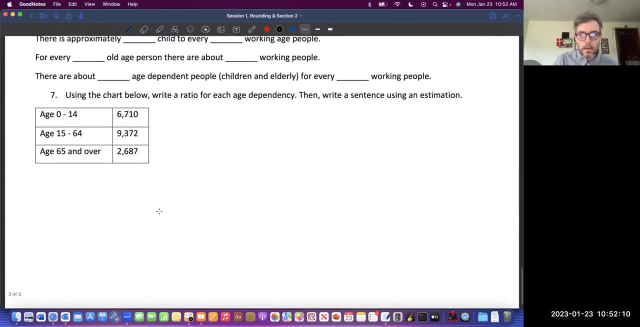 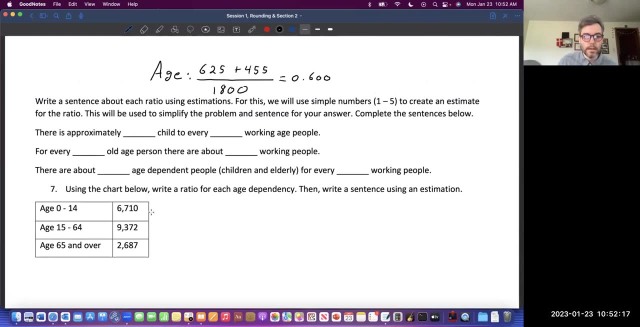 Okay, But thank you, That was a little confusing. I don't think I said that. Okay, Let's see, I have eight minutes. If it's okay with you, I'm just going to skip Right to the, Because I'm almost out of time. All right, Let's do it again. So we're going to. 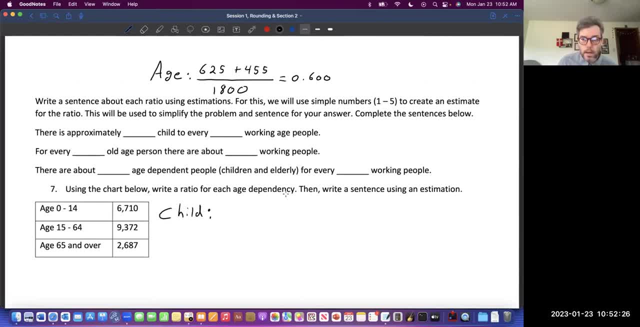 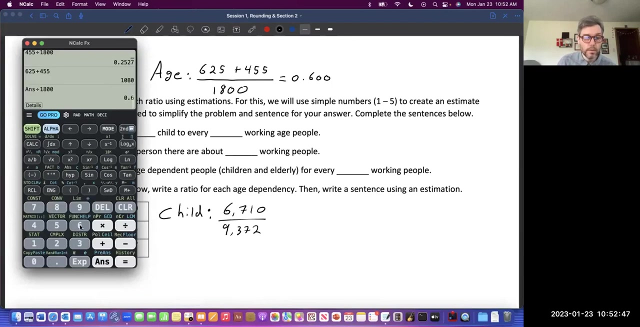 do the child dependency ratio, And here we are going to write the ratio, write a ratio for each dependency and then use a sentence using an estimation: Okay, 6,710 over the working age, 9,370.. If we can, we would like to reduce. 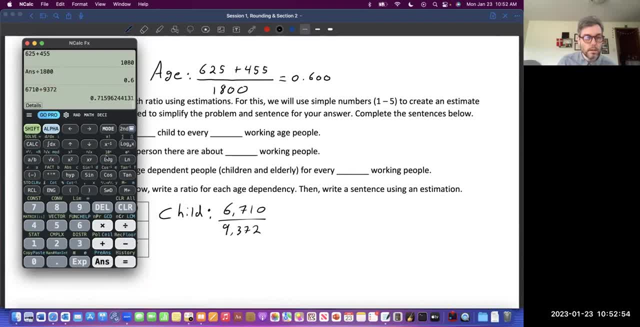 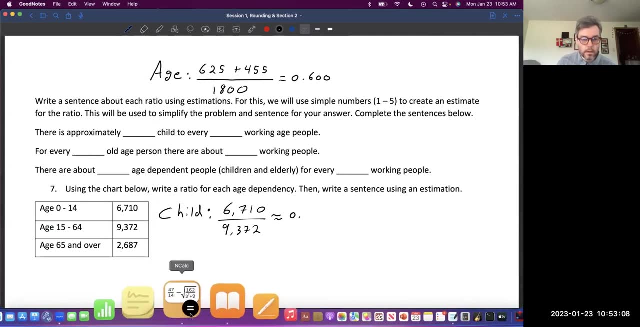 9,372.. Does this reduce Not really? Okay, Not really. Now we can use an estimation: It's approximately 0.716.. 1, 2, 3, 4, 6, 5, Okay saying let's get together 2,680.. 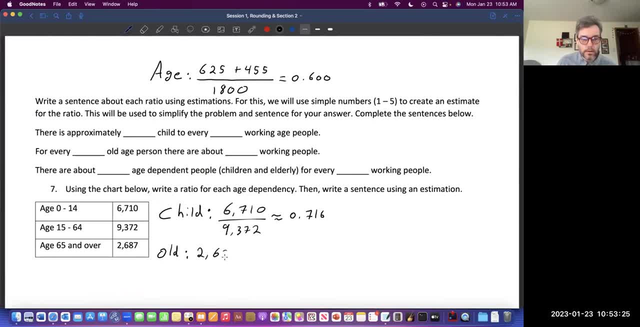 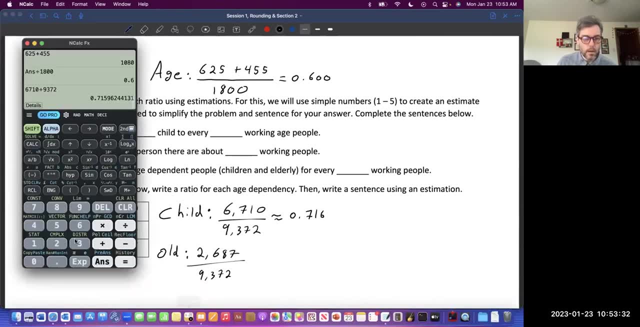 Okay, The old age dependency ratio is the 2,687 divided by the working. Okay, 2,687 divided by 9,372.. I think I plugged that in right. 2,687, 9,372. is approximately two eight seven. 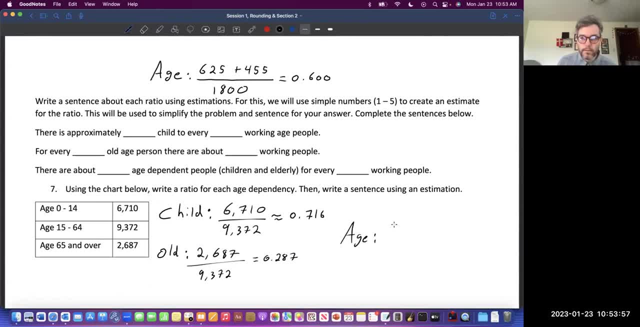 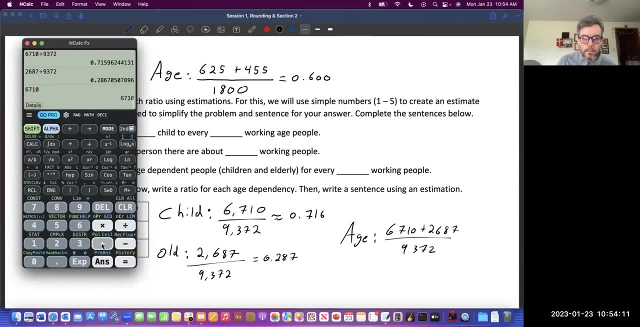 And then the age dependency ratio is both of them. Okay, so let's do that: Six, seven, 10 plus two, six, eight, seven Divided by nine, three, seven, two, Oh, oh, oh, did I mess up? 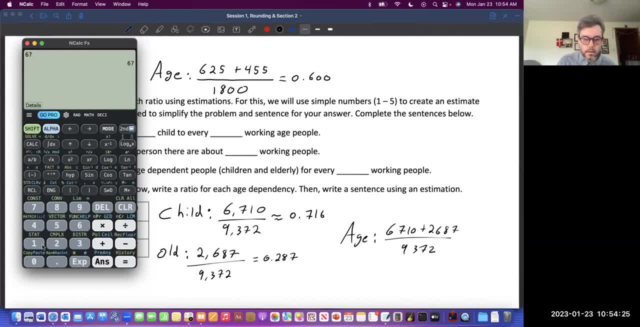 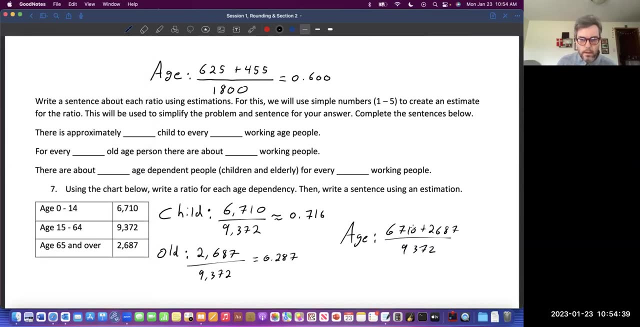 I think I did And maybe I heard someone's voice. Was there a question? Two, six, eight, seven- I wrote something down wrong- Six, seven, 10,. two, six, eight, seven, nine, three, seven, two.